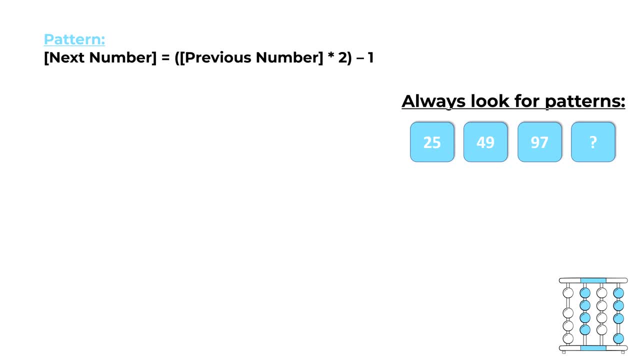 is calculated as previous number multiplied by 2 minus 1.. So for example, first number 25 is the given, but the next number, 49, is calculated as 25 multiplied by 2 minus 1, which equals 50 minus 1, which equals 49.. 97 is calculated 49 multiplied by 2, equals 98, and 98 minus 1 equals. 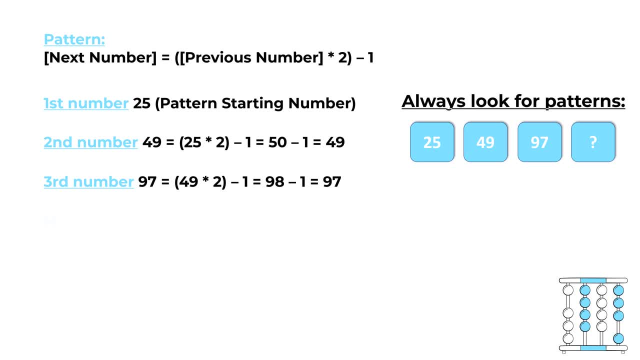 97.. So the correct answer here is calculated as 57 multiplied by 2 minus 1, which is equivalent of 194 minus 1, and the end result of this is 193.. So the correct choice here is choice D, 193.. Hopefully you've nailed this question. and now, 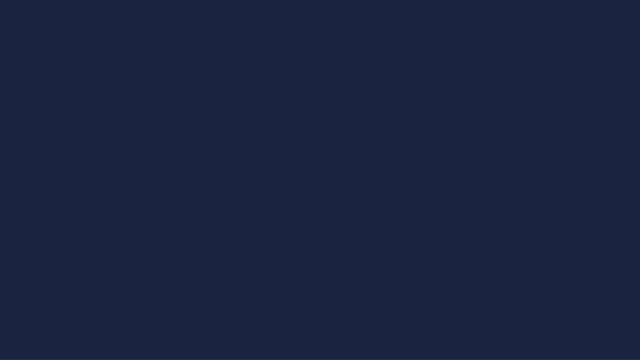 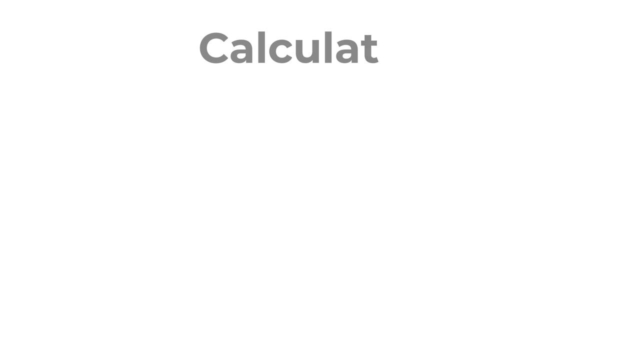 know how to answer similar problems on the test. Here's a cool question you frequently see on the test. You need to calculate the question mark And you're presented with the three-layer pyramid and the bottom layer you have numbers eight and two. On the middle layer you have numbers four and six And in the 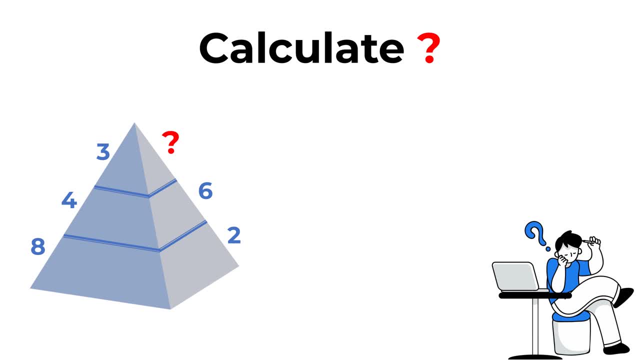 top layer you have numbers three And on the other side of the pyramid you have a question mark, And this question mark can be one of those four values. Your choice A is six, choice B is 10, choice C is seven and choice D is two. Do you see the answer? Give yourself a little bit of time. 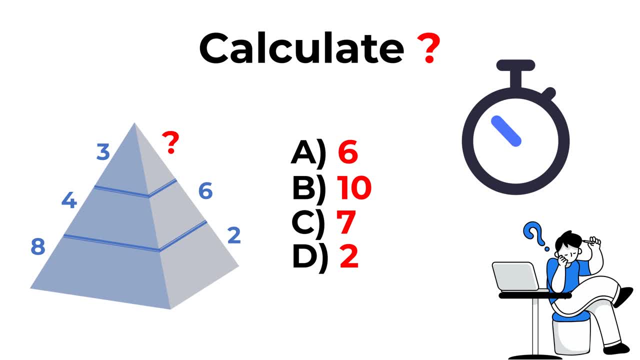 For some of you, this type of question might be easy, But for some of you it might require some thinking. So feel free to pause this video to see if you can come up with the solution. Ready or not, let's go ahead and get to the correct solution together. 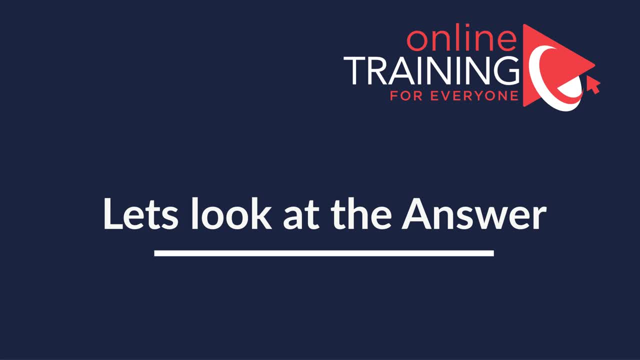 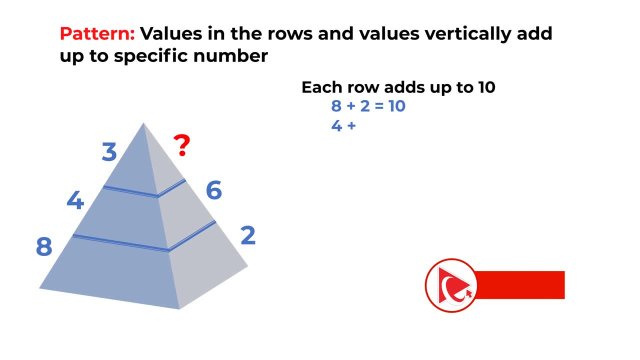 As you might have figured out, the key to solve these types of challenges is always look for patterns, And if you look closely, each row adds up to 10. And vertically, values also add up to 15.. So the correct answer here is choice C seven. Hopefully you've nailed this question. and now, 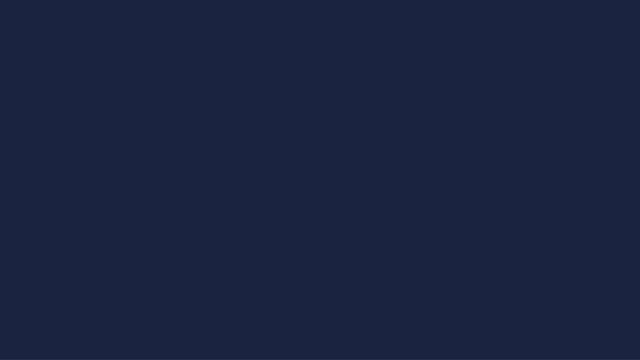 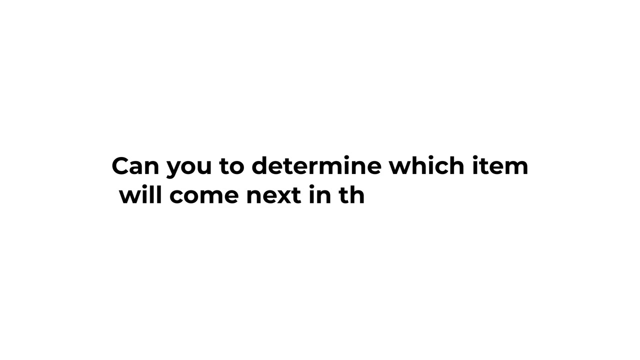 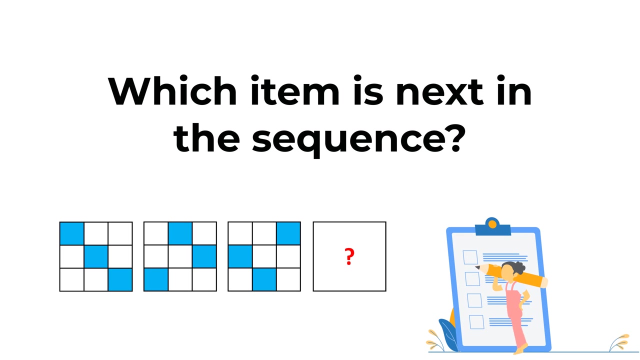 know how to answer similar problems on the test, And now I have a practice question for you. You need to determine which item comes next in the sequence. You're presented with three large squares. Each large square contains nine small squares inside, And small squares are of a 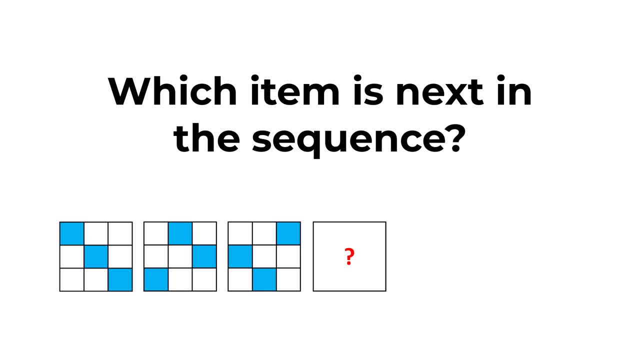 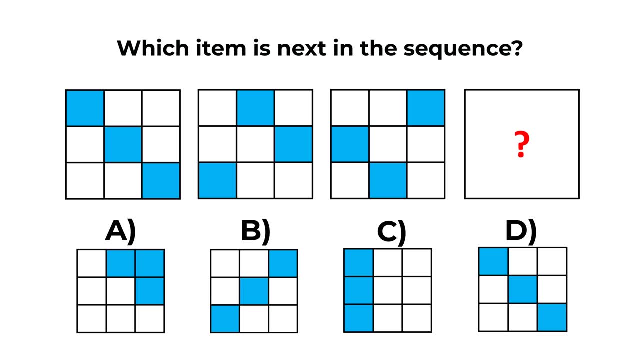 different color And the fourth square is missing And you have four different choices to choose from: Choices A, B, C and D. Do you see the answer? Give yourself 10 to 15 seconds to see if you can come up with the solution And make sure to post. 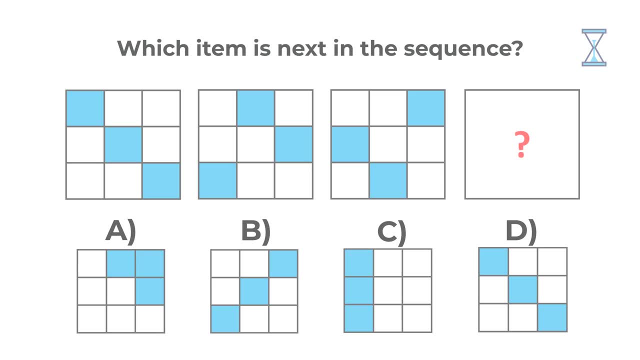 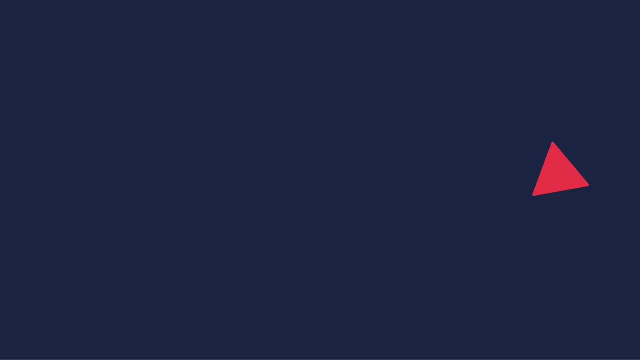 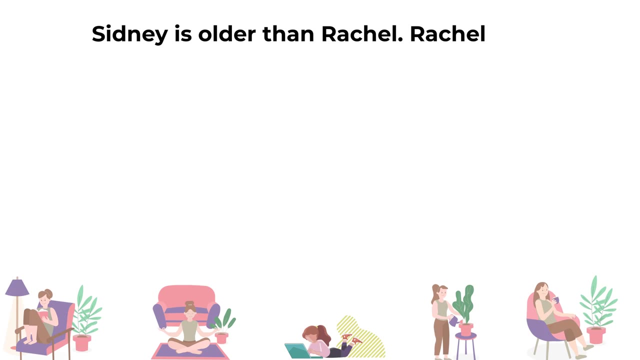 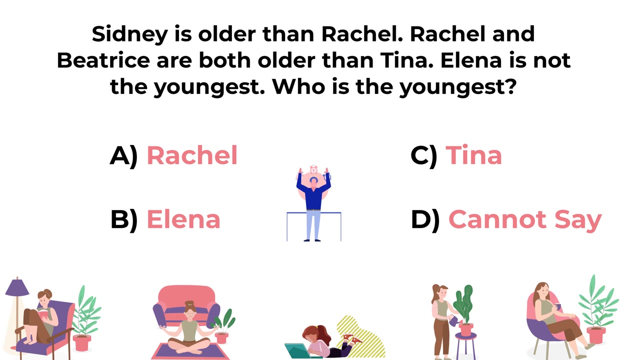 your solution and your rationale in the description section of this video. This way, I can give you my feedback. Thanks for participating and good luck. Here's one of the questions we frequently see on the test. Do you see the answer? Give yourself a little bit of time to see if you can come up with the solution. 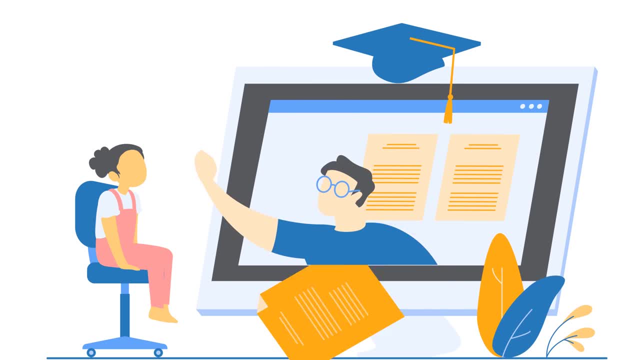 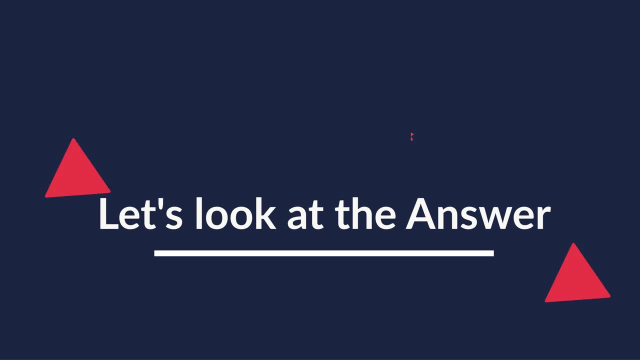 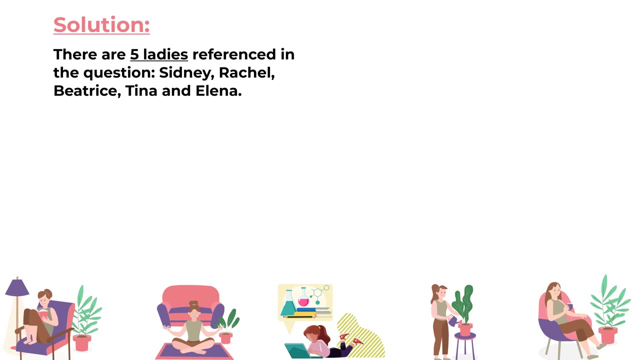 Ready or not, let's move forward and get to the correct solution. To solve these types of challenges, you need to look at the facts as well as look at the common sense. There are five ladies referenced in this question: Sydney, Rachel, Beatrice, Tina and Elena. Sydney is older than Rachel, So obviously Sydney is not the youngest. By the same logic, neither Rachel nor Beatrice are the youngest, Because Tina is younger than both of them. That leaves Tina and Elena. And the answer is B, The answer is C, The answer is C. The answer is C. 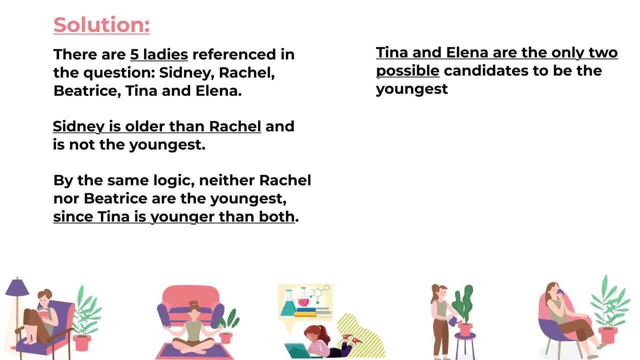 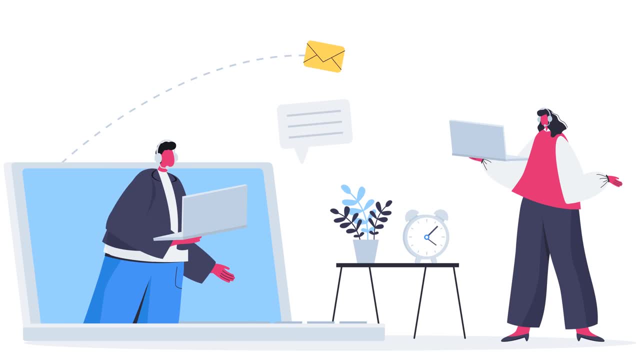 But the last sentence in the question mentions that Elena is not the youngest. So, based on this rationale, Tina is the youngest, So the correct choice here is choice C: Tina is the youngest. Hopefully you've nailed this question and now know how to solve similar problems on the test. 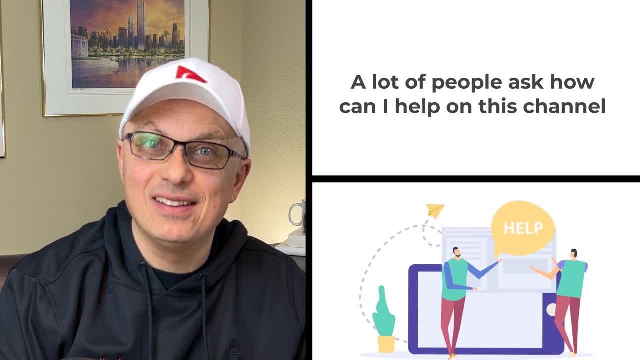 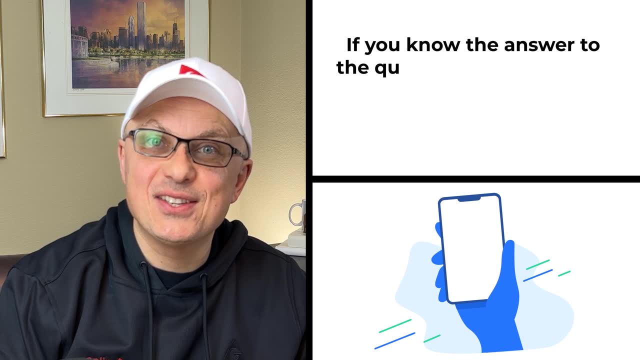 A lot of people ask: how can I help on this channel? One of the best ways to help is to help other people answer the questions that they are getting. If you know the answer to the question you see in the comments, please post the answer in the. 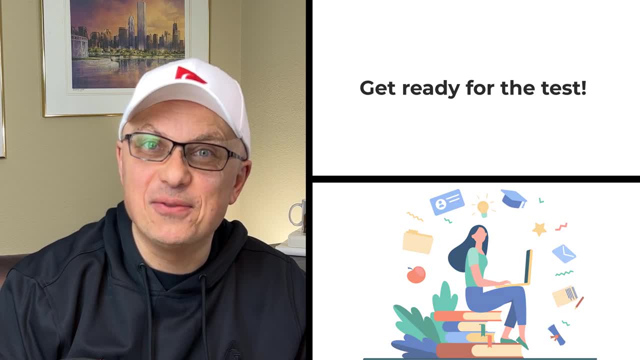 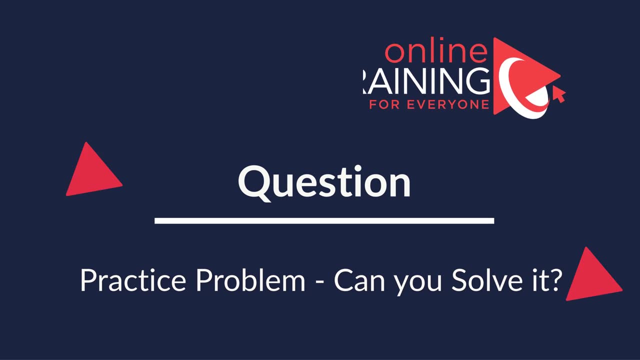 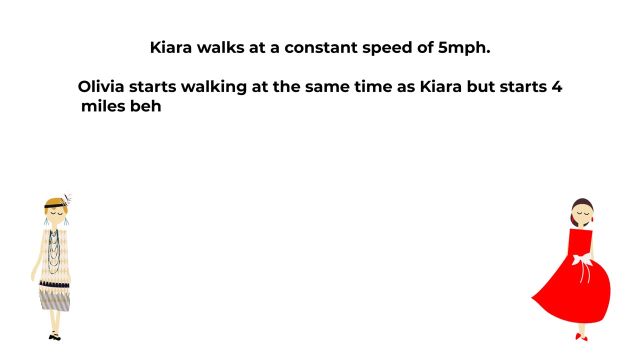 comment section of this video. And now let's continue and get you ready for the test. Here's the practice question for you. Chiara walks at the constant speed of five miles per hour. Olivia starts walking at the same time as Chiara, but starts four miles behind her. 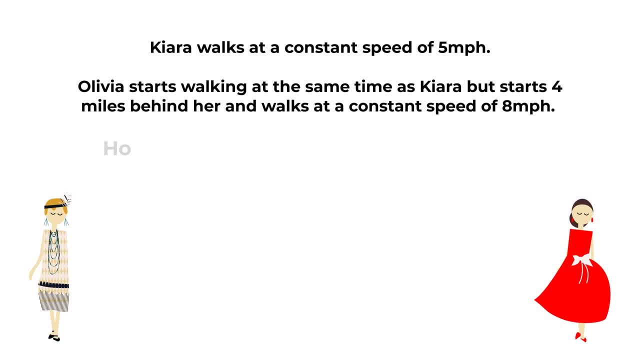 and walks at the constant speed of eight miles per hour. How long will it take Chiara to catch up with Olivia? And you have four different choices: Choice A- 50 minutes, Choice B- 60 minutes, Choice C- 70 minutes And then choice D- 18 minutes. Please give yourself a little bit. 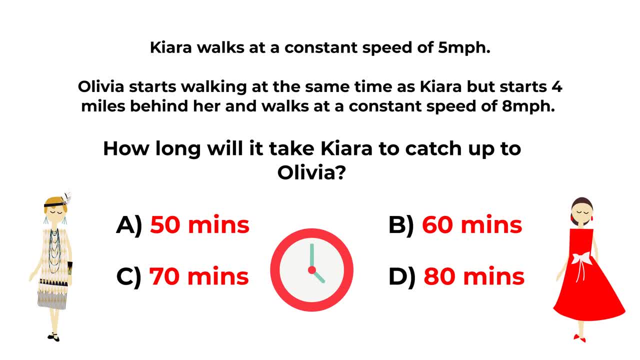 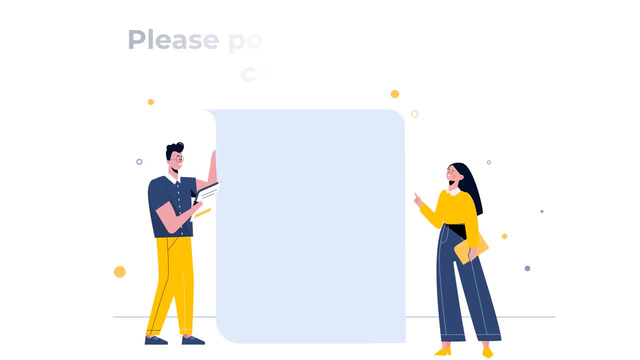 of time to see if you can come up with the solution. The answer to this problem is not obvious, But if you came up with the solution, please make sure to post it in the comment section of this video so I can give you my feedback. Thanks for participating and good luck. 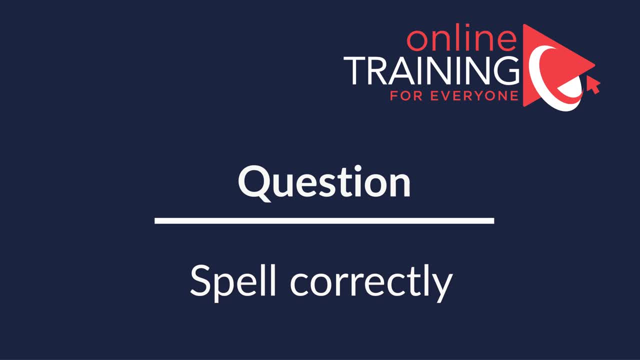 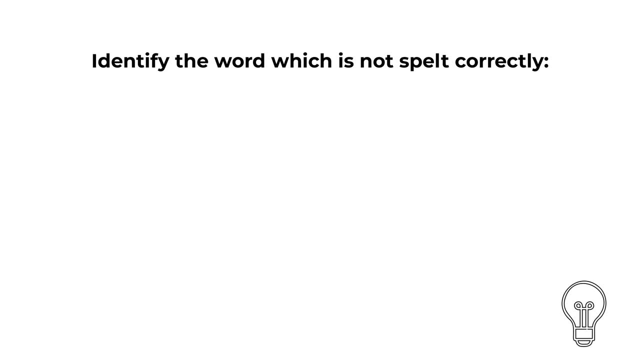 Here is the spelling question Which we frequently see on the test. You need to identify the word which is not spelled correctly And you are presented with four different words: Choice A- hypothetically. Choice B- accommodation. Choice C- incomprehensibilities, And choice D- interdisciplinary. Do you see the answer Give? 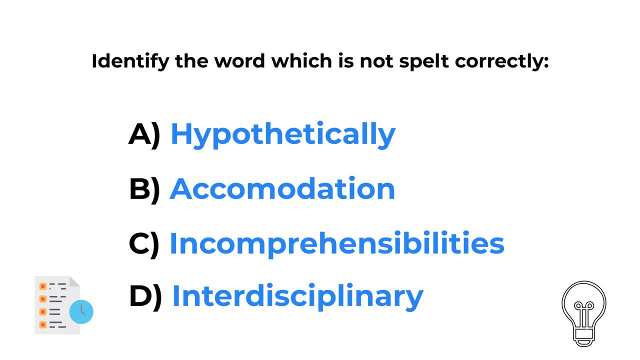 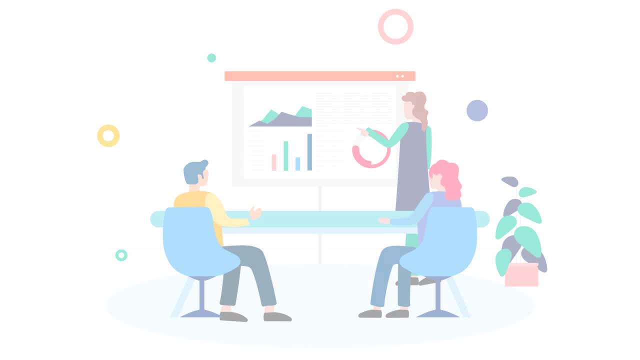 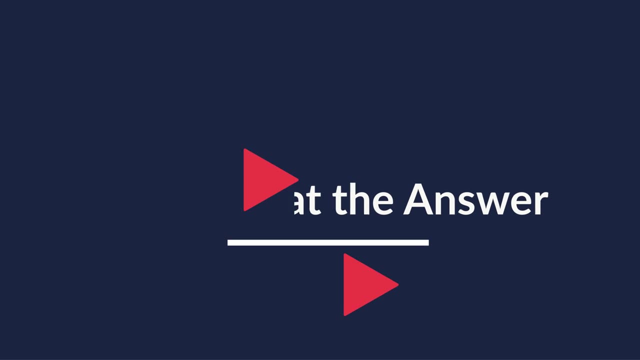 yourself a little bit of time so you can browse through words and see if you can come up with the correct solution. Ready or not, I am going to move forward and explain you the correct solution to this problem. As you must have figured out, the correct answer here is choice B And the correct spelling for: 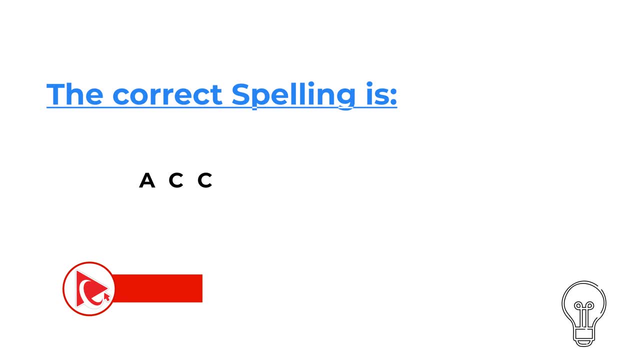 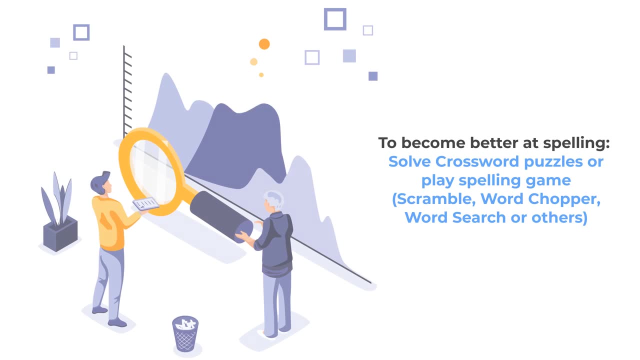 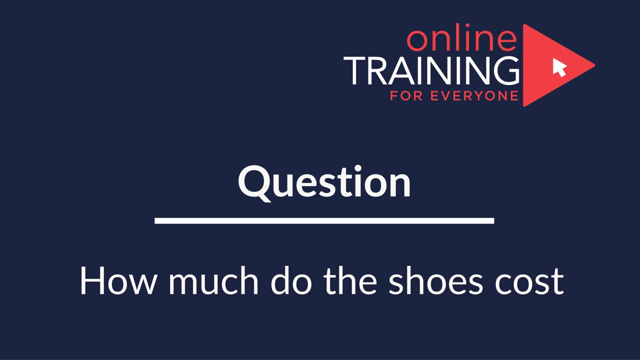 the word accommodation is A-C-C-O-M-M-O-D-A-T-I-O-N. Hopefully you nailed this question and now know how to answer similar problems on the test. Here is the cool question that you frequently get in the test. kate has 33 dollars, which is only 20 of the cost of shoes that she would like to. 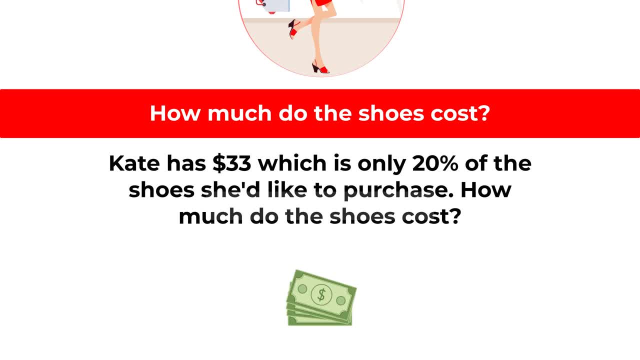 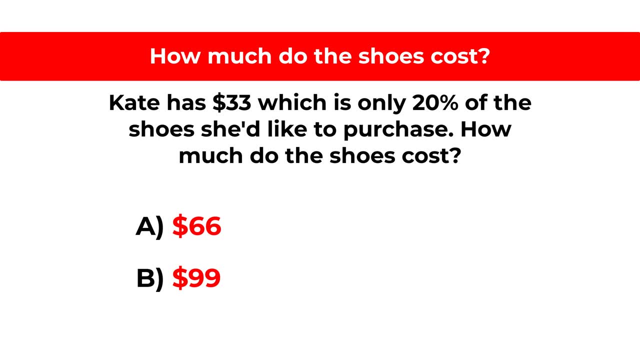 purchase. how much do the shoes cost? and you're presented with four different choices: choice a- 66 dollars, choice b- 99 dollars, choice c- 150 dollars and choice d- 165 dollars. can you calculate the answer? give yourself 10 to 15 seconds, maybe 20 to 30 seconds, depending how well you are with. 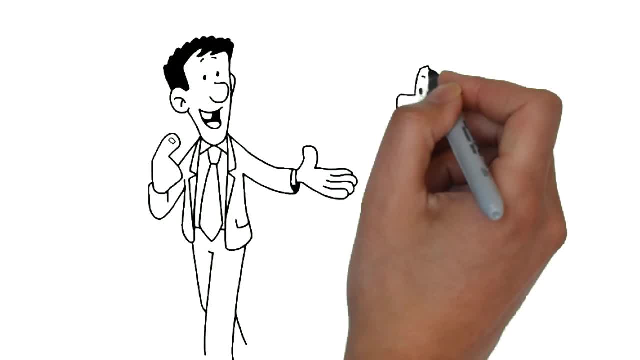 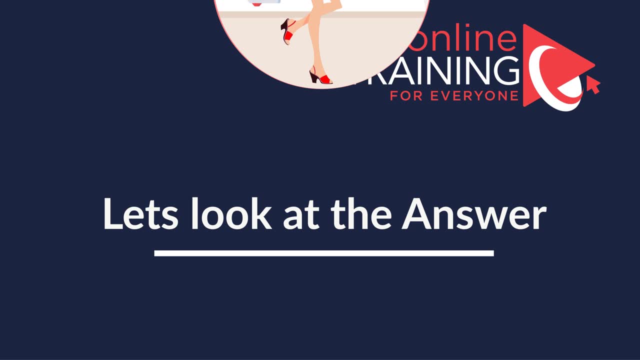 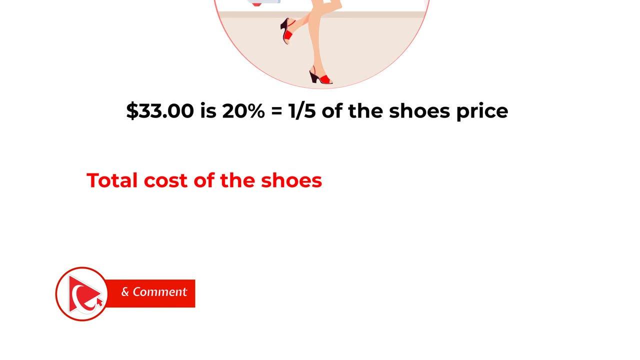 math and percentages. ready or not, let's go ahead and get to the correct solution together: the. the answer to this problem is very simple. 33 is 20 percent, or one-fifth, of the shoes price. so the total cost of the shoes would be 33 multiplied by 5, which would be equal 165 dollars. 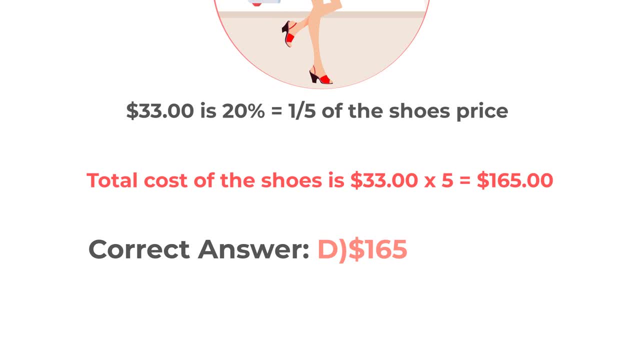 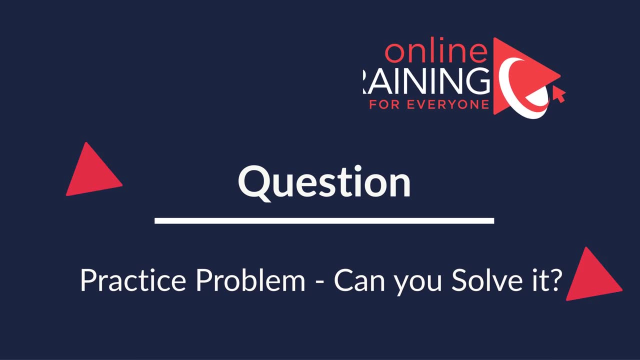 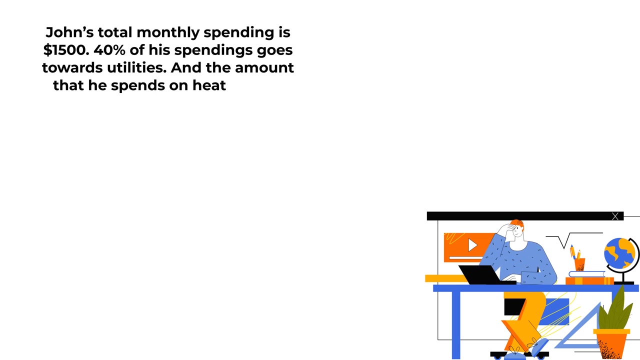 so the correct answer here here is choice d, 165 dollars. here's an interesting question. you might easily get on the test. john's monthly spending is fifteen hundred dollars. forty percent of his spending goes toward utilities and the amount that he spends on heating and electricity is fifteen percent more than what. 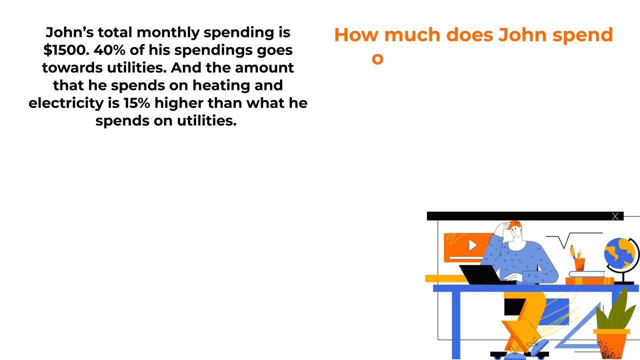 he spends on utilities. how much does john spend on things besides heating, electricity and utilities? you're presented with four different choices: choice a- 210 dollars, choice b- 220 dollars, choice c- 230 dollars and choice d- 240 dollars. do you see the answer? give yourself a little bit of time to see if you can calculate. 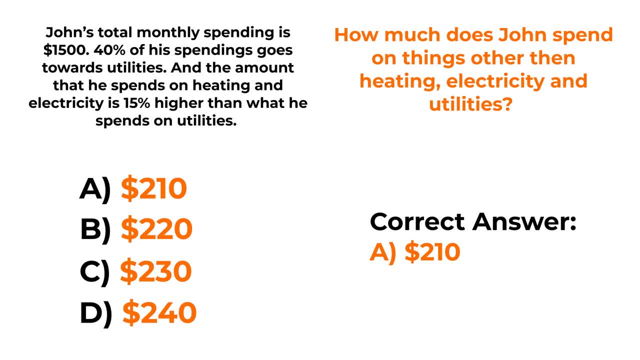 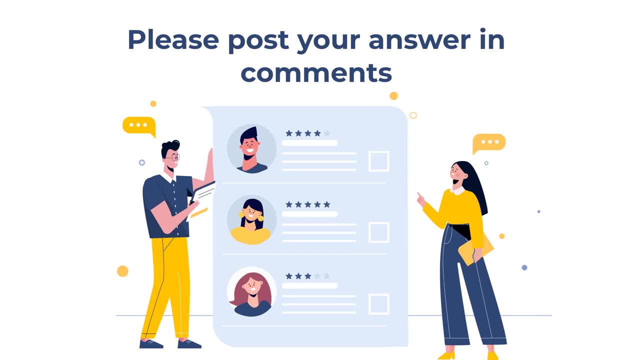 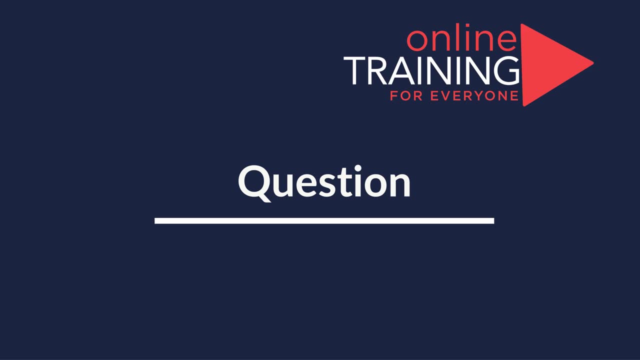 the solution. the correct answer here is choice a: 210 dollars. do you know how to get to this answer? if you figured it out, please make sure to post your answer in the comment section of this video, and good luck. here's the cool question that you frequently get on the test you're presented with. 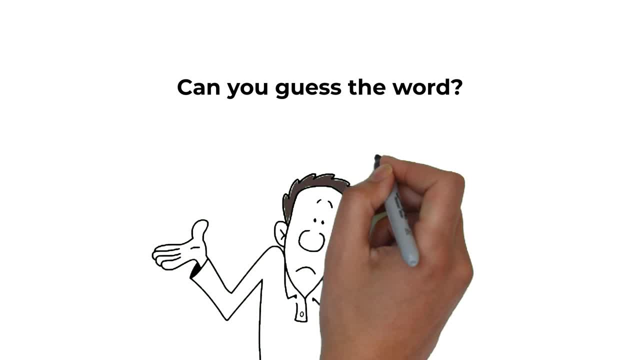 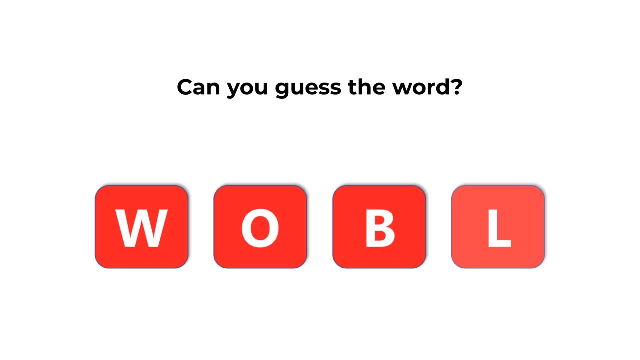 four different letters and you need to guess the word using all letters presented. the letters we have are w, o, b and l. can you guess the word? give yourself 10 to 15 seconds to see if you can come up with the answer, ready or not, let's go ahead and reveal the solution. 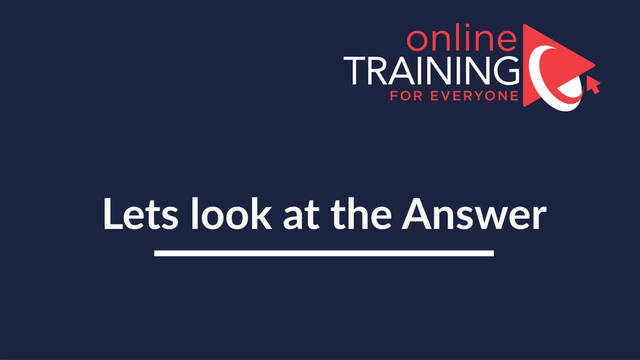 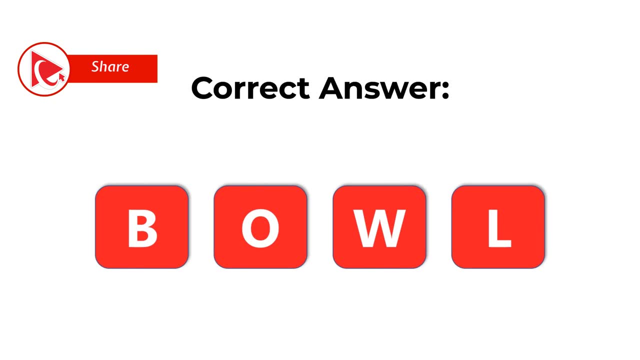 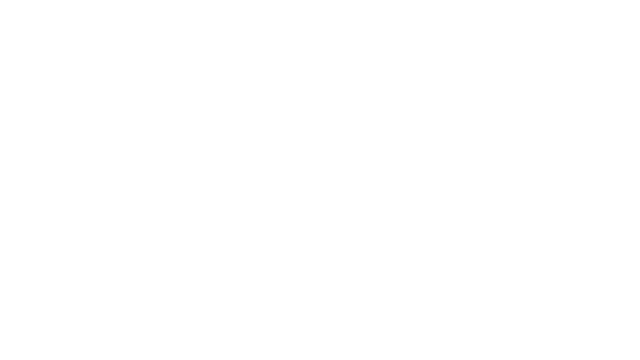 the correct answer here is ball, which is spelled as b o, w and l. hopefully you've nailed this. the correct answer here is ball, which is spelled as b o, w and l. hopefully you've nailed this question and now know how to answer similar problems on the test. i would like to ask you. 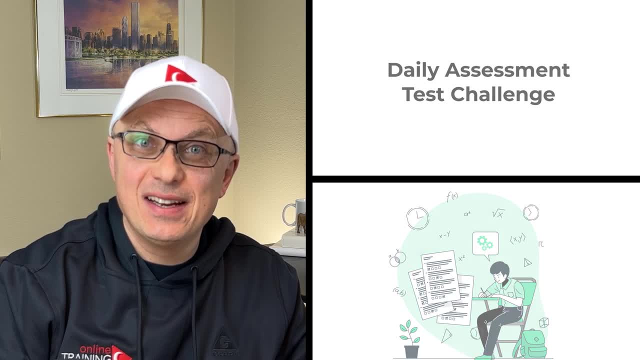 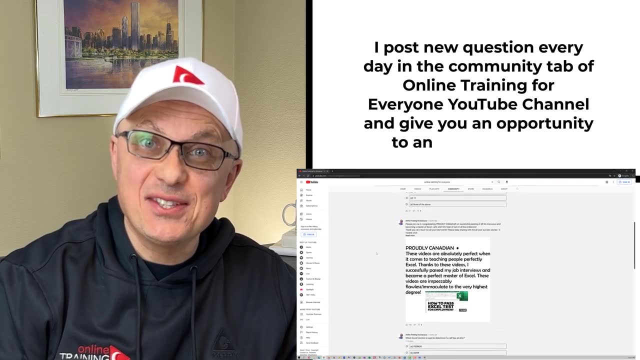 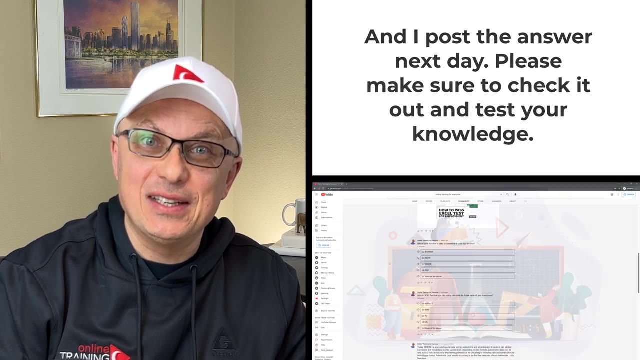 to participate in our daily assessment test challenge. i post new question every day in the community tab of youtube channel and give you an opportunity to answer it in. try it and i post answer in comments next day. so please make sure to check it out to test your. 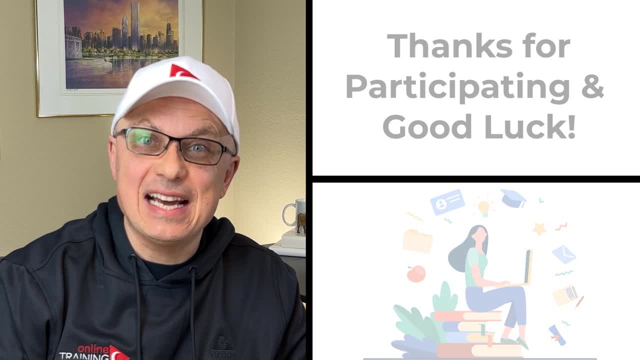 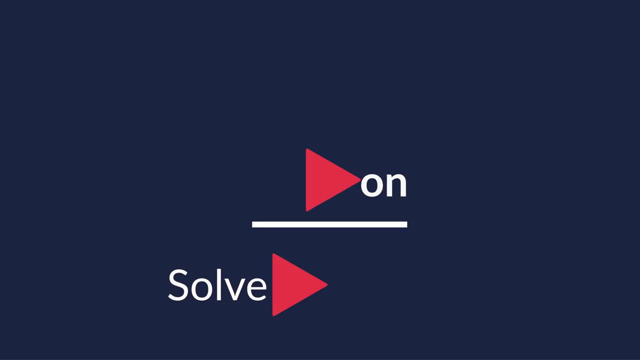 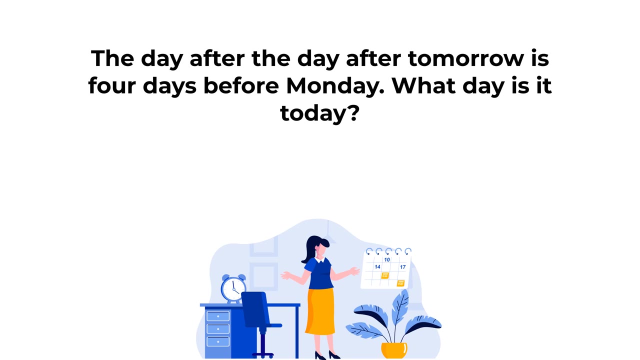 knowledge. and now let's continue and get you ready for the test. here's the cool question which tests your ability to quickly come up with the answers the day after. the day after tomorrow is four days before monday. what day is it today? and you have four different choices: choice a- sunday. choice b: 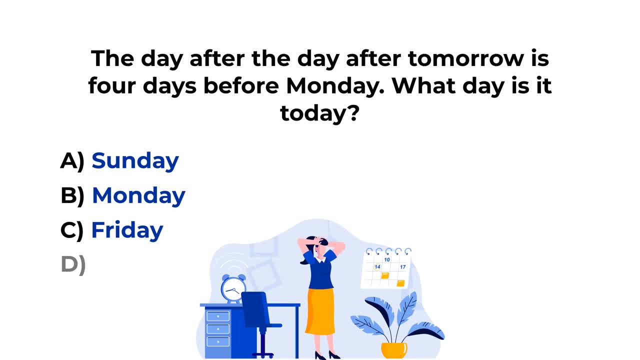 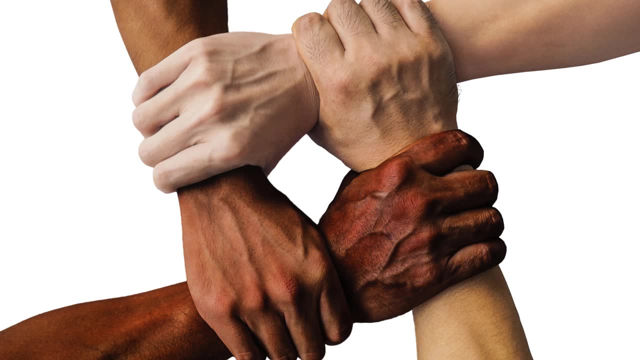 monday. choice c- friday and choice d- saturday. do you see the answer? think again. these types of puzzles might require you to do some thinking, so feel free to pause this video to see if you can come up with the answer, ready or not. i am going to move forward and get us to the correct. solution together. to solve these types of problems, we need to analyze them and do them in reverse: four days before monday is thursday and the day before day before thursday is tuesday. if tomorrow is tuesday, it means that today is monday. so the correct answer here is choice b- monday. hopefully you've nailed this question. 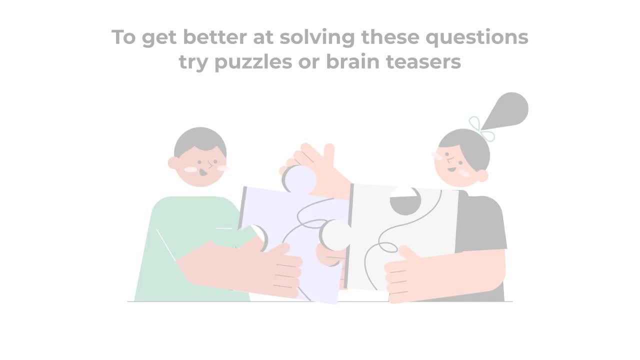 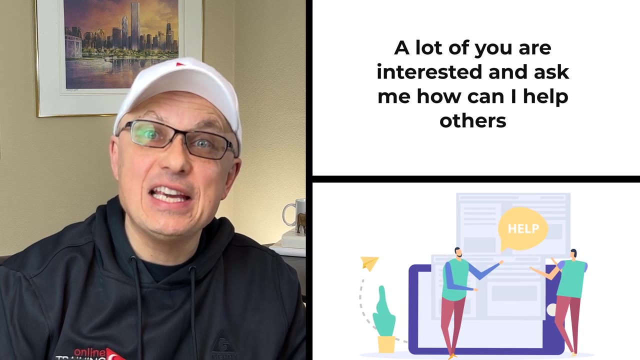 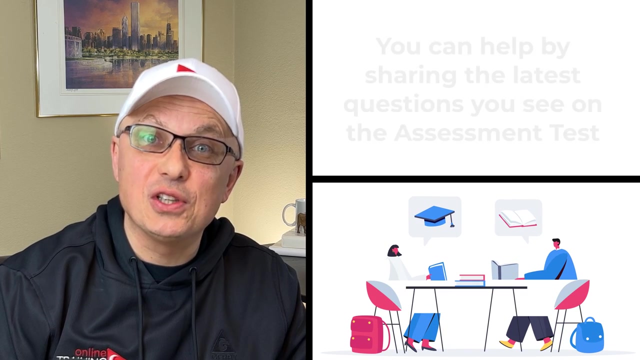 and now know how to answer similar puzzles on the test. a lot of you are interested and ask me: how can i help others? one of the ways you can help other people is by sharing the latest questions you see as part of the assessment test, and when you share, please make sure to also include how. 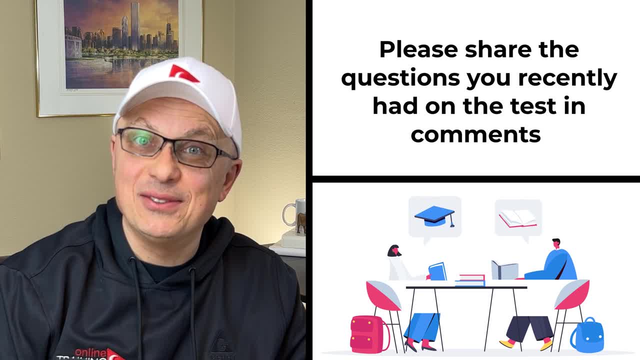 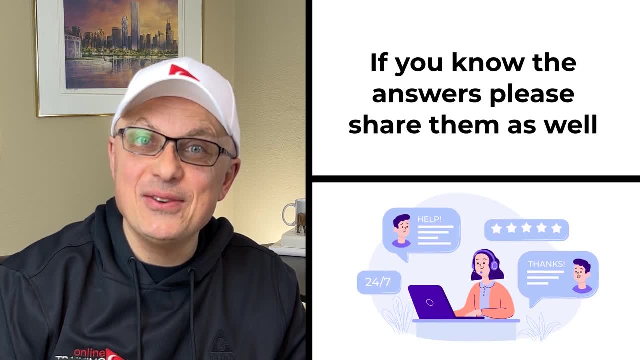 you answered them. please share the question you recently encountered in the comment section of this video and if you know the answers, please share them as well. and now let's continue and get you ready for the test. here's the puzzling question that you might frequently see on the test. 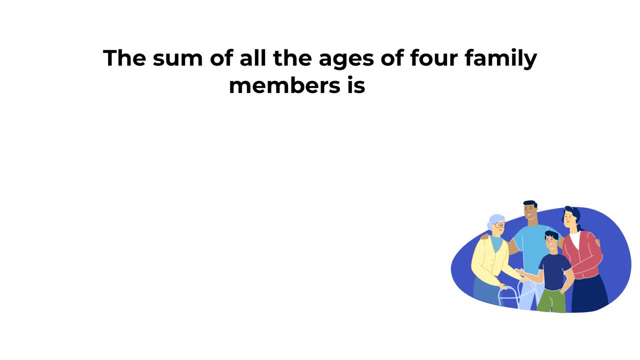 the sum of all the ages of four family members is 85. what would be the sum of their ages together in five years? and you're presented with four different choices: choice a- 90, choice b- 95, choice c- 100 and choice d- 105. do you see the answer? give yourself 20 to 30 seconds. 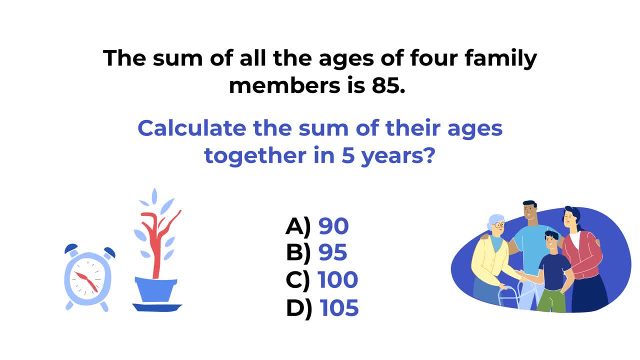 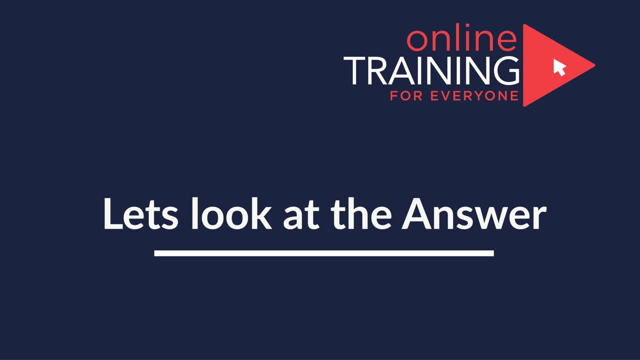 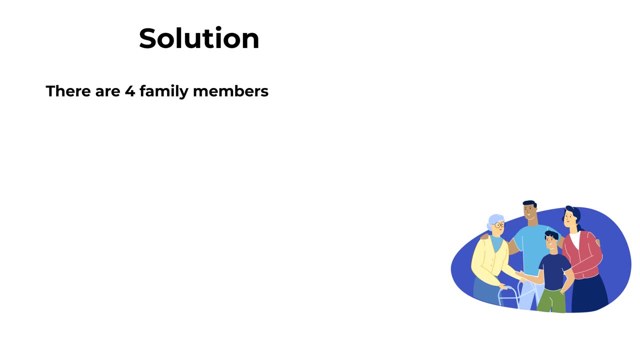 to see if you can come up with the solution ready or not. i'm moving forward to get to the correct solution together. what's interesting about this problem is that it is simpler than you think, so the key here is not to overthink the problem. there are four family members and some of the 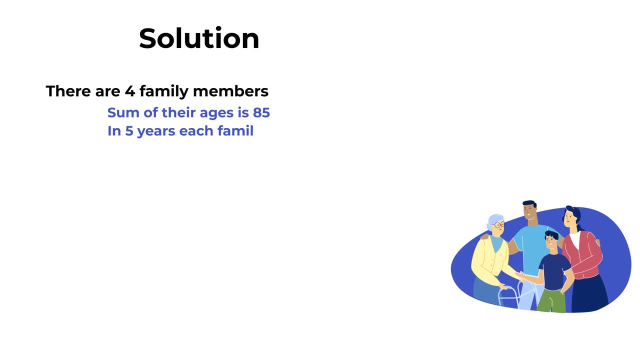 ages is 85 and in five years each family member will be five years older. so incremental age increase for all family members can be calculated as four. four family members multiplied by five. five years equals 20 years. so some of the ages of all family members in five years can be calculated. 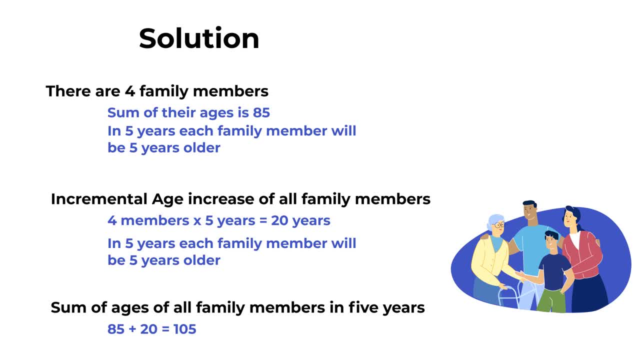 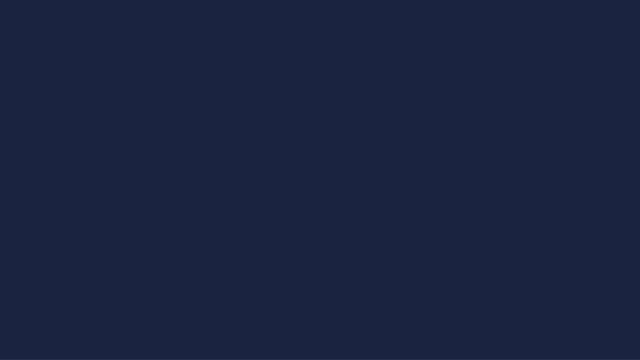 as 85, which is original sum plus 20, which is the incremental age increase, and would be equal to 105.. so the correct choice here is choice d, 105.. hopefully you've nailed this question and now know how to answer similar puzzles on the test. and now here's the question for you to practice. 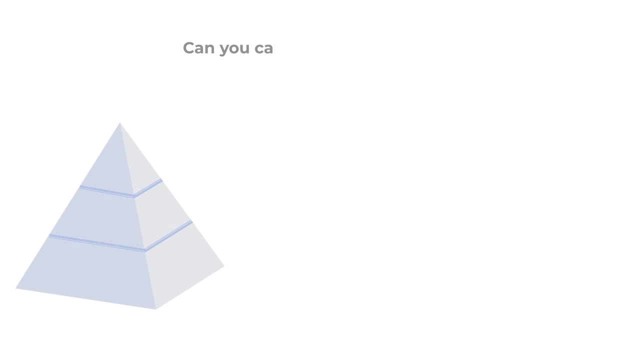 you're presented with triangle which is broken down into three equal horizontal parts. on the left side of the triangle, you see numbers eight, four and three if you go from the bottom to the top, and on the right side of the triangle, you see numbers eight, four and three if you go from the bottom to the top and on the right side of the. 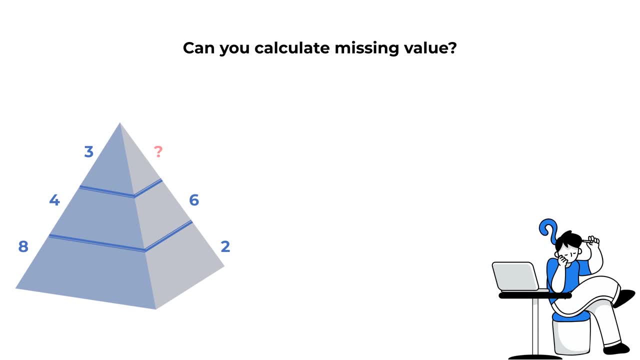 triangles you see numbers two, six and one number is missing. you need to select missing number from four different choices: choice a, 6, choice b, 10, choice c, 7 and choice d, 2. give yourself a little bit of time to see if you can come up with the solution. if you figured out the solution, please 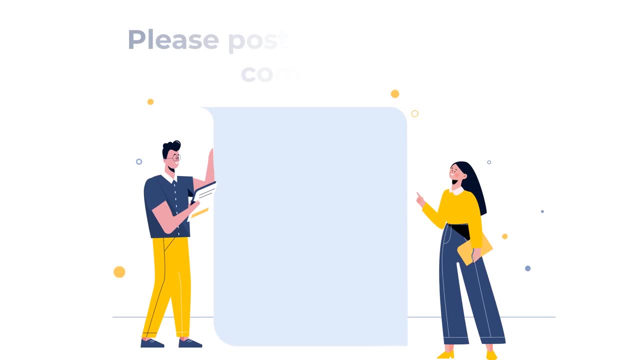 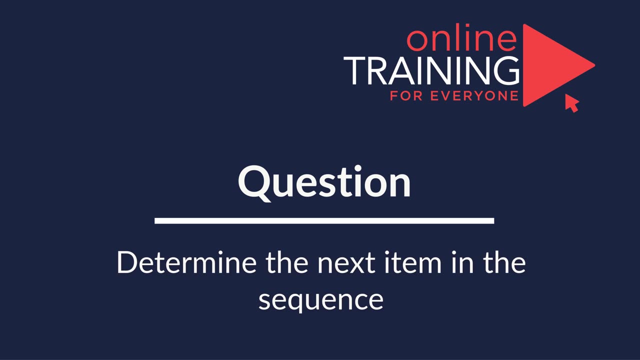 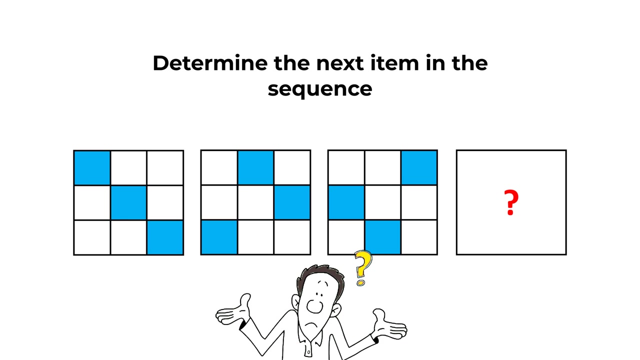 make sure to post your answer in the comment section of this video so i can give you my feedback. thanks for participating and good luck. here is a very interesting problem that you might frequently get on the test. you need to determine the next item in the sequence. you're presented with the sequence of large squares. each large square contains nine small squares. 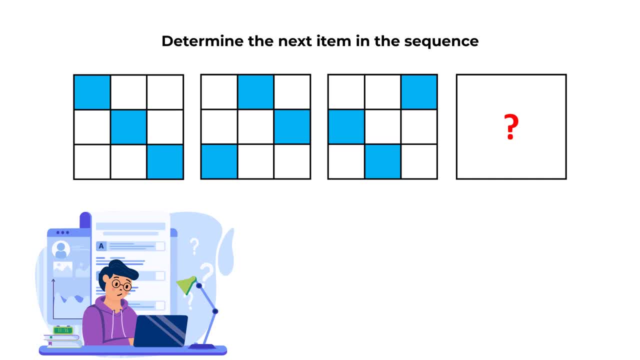 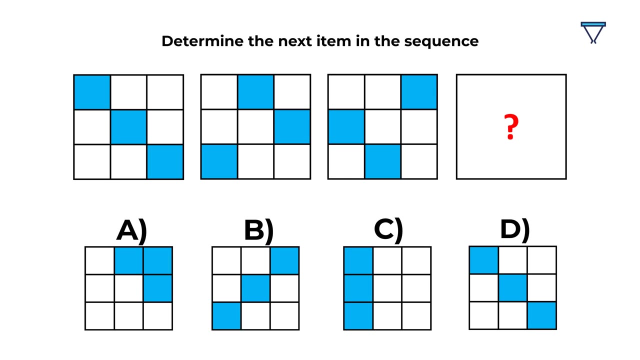 inside and small squares are of the different color. you need to determine next item in the sequence and you have four different choices: choices a, b, c and d. do you see the answer? give yourself 10 to 15 seconds, maybe longer, maybe 20 to 30 seconds, to see if you can come. 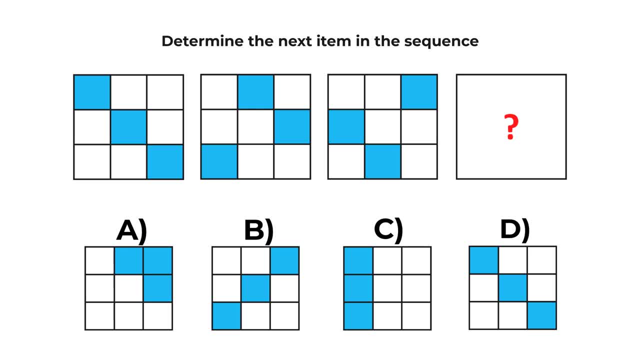 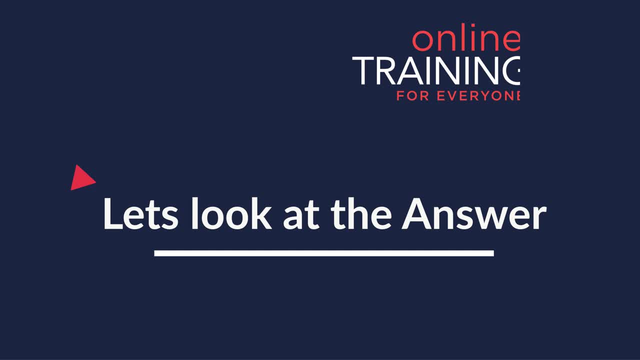 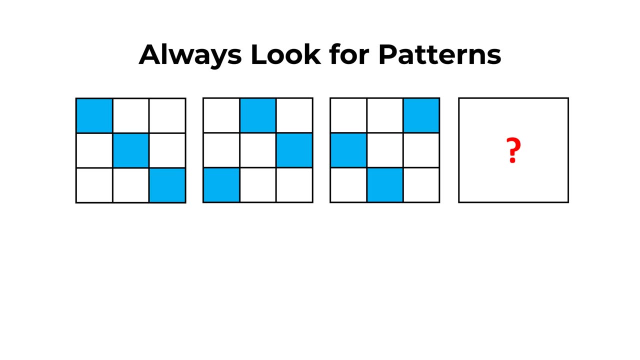 up with the solution. did you figure it out? let's go ahead, move forward to get to the correct solution together. as always, my advice to you: look for patterns, and determining the pattern is key to solving this particular problem. what you need to know to answer this particular question. 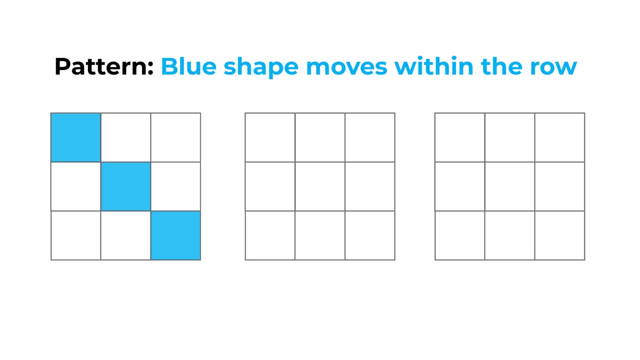 is that blue shape moves within the row of the larger shape. in each row, blue shape moves from left to right, one step at a time, and once blue shape reaches the end of the row on the right, it reappears on the left. so the correct answer here is choice d. hopefully you've. 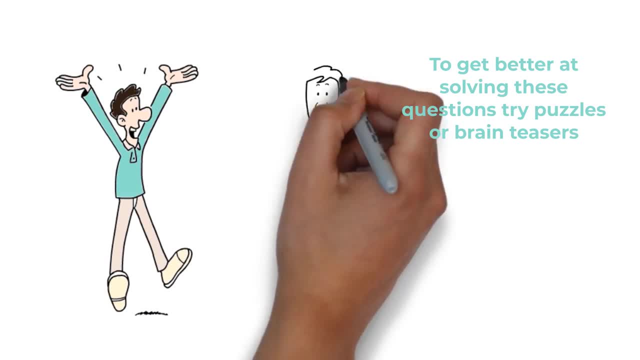 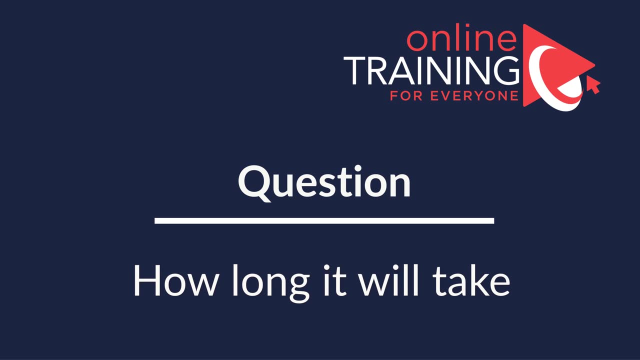 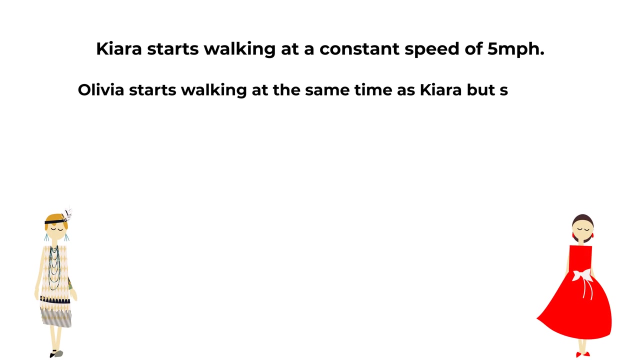 nailed this question and now know how to answer similar problems on the test. here's an interesting question we frequently see on the test. kiara walks at the constant speed of five miles per hour. olivia starts walking at the same time as kiara, but starts four miles behind. 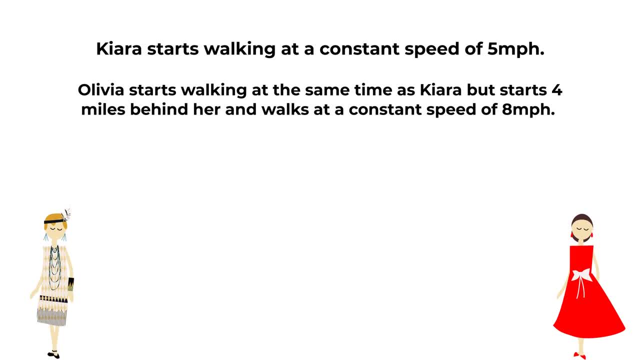 her and walks at a constant speed of eight miles per hour. how long will it take for kiara to catch up with olivia? you're presented with four different choices: choice a- 50 minutes, choice b- 60 minutes, choice c- 70 minutes and choice d- 80 minutes. do you see the answer? give yourself a little bit of time. 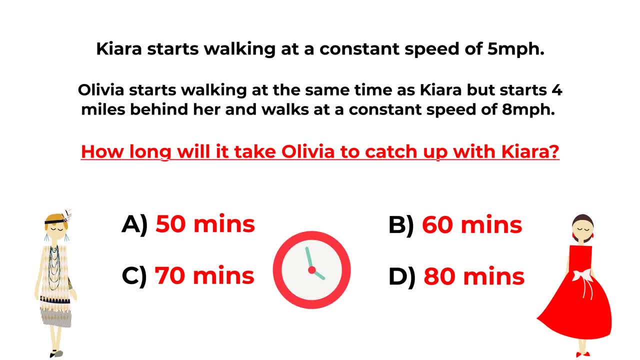 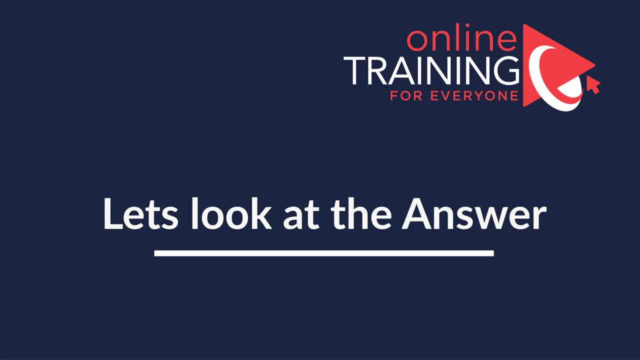 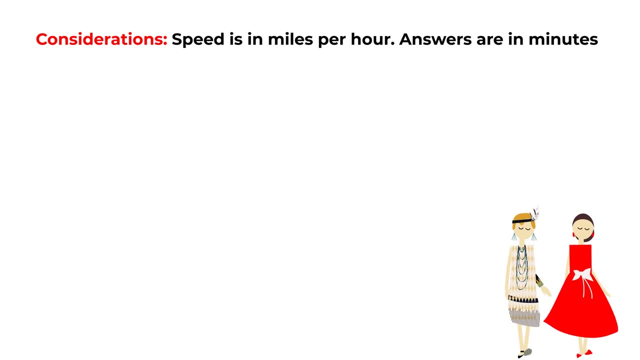 all possible combinations. ready or not, let's move forward and get to the correct solution together. one important consideration to help you solve this challenge is that the speed for both kiara and olivia is presented in miles per hour, but answers are in minutes, so at some point we would need to make a conversion. another important 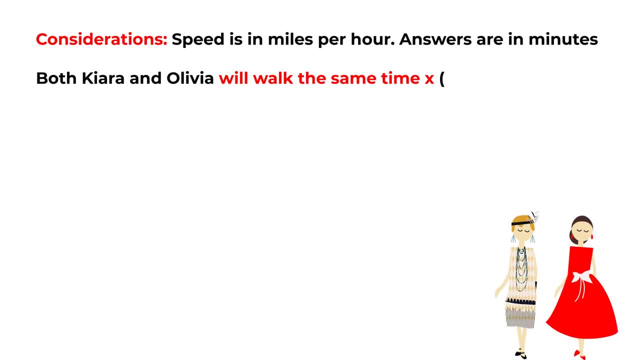 point is that both kiara and olivia will walk the same time and we can put it as x in hours before catching up, because they started at the same time. in our solution, x will be the time in hours when they will catch up, and me. to solve this challenge, we need to build an equation. 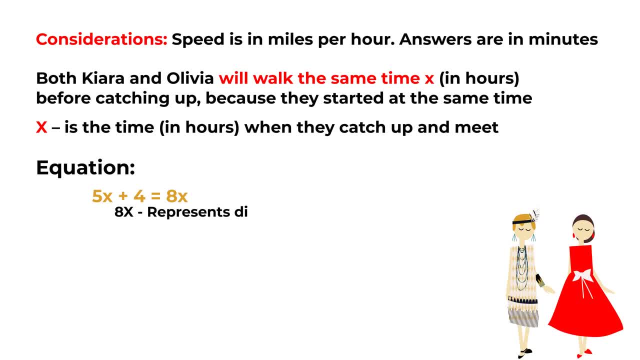 5x plus 4 equals 8x. 8x represents how much olivia will walk, and 5x plus 4 is representing how much kiara can walk, and the starting point for this will be starting point of where olivia starts, since olivia starts four most times. 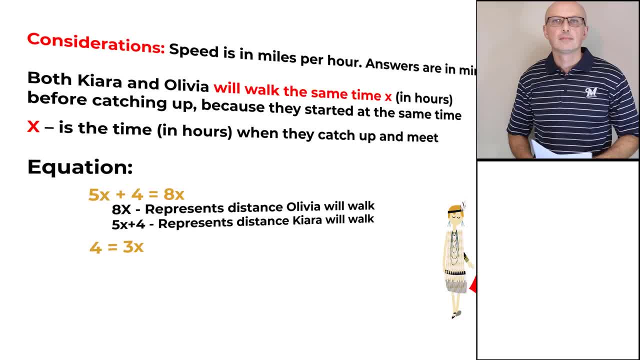 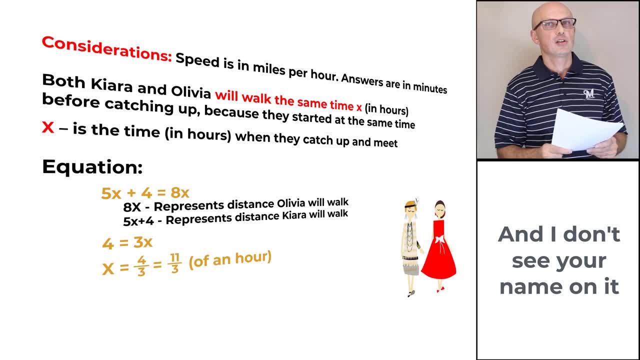 miles behind. So if we simplify this equation, 4 will be equal to 3x And x will be equal 4 thirds, or 1 and 1 third of an hour. And now is the time to do the conversion: 1 hour equals 60 minutes.